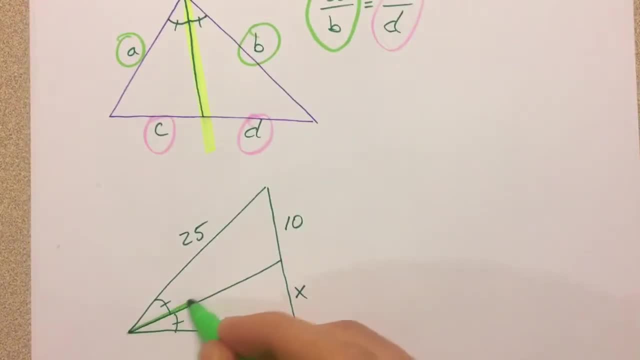 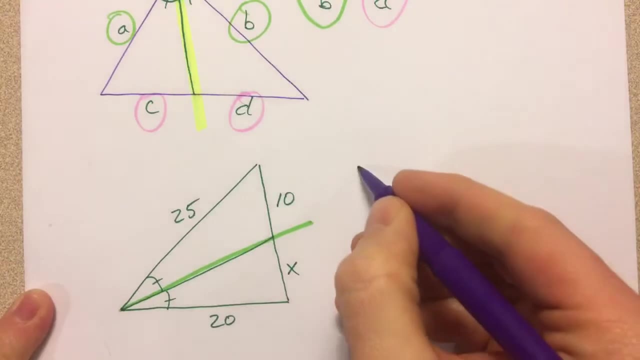 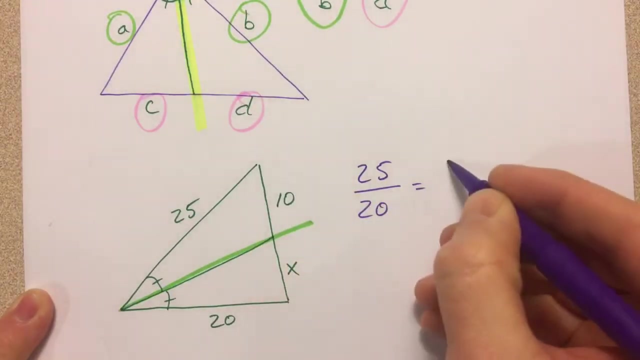 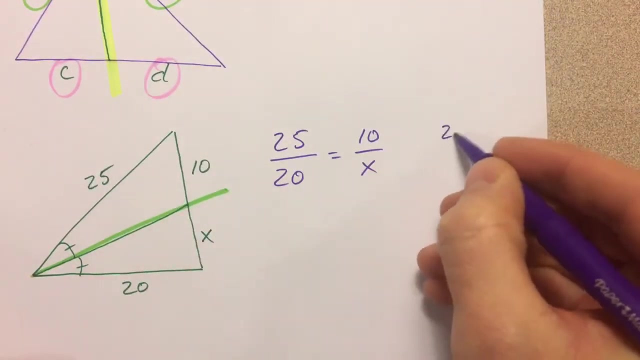 We've got this angle bisector cutting through, and so I compare both sides of the angle bisector to each other, So I can compare the 25 to the 20, and I can compare the 10 to the X. Now you could also compare the 25 to the 10, and the 20 to the X. 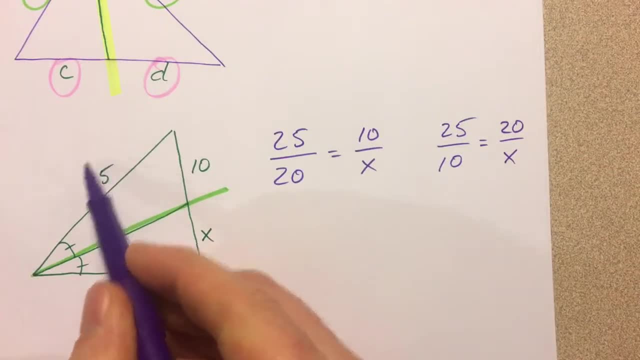 The idea is that we're comparing the pieces that are corresponding to each other, And so the two sides of the triangle, and then the two pieces formed by the angle bisector, this angle bisector cutting through. So then, how we solve our proportions again. 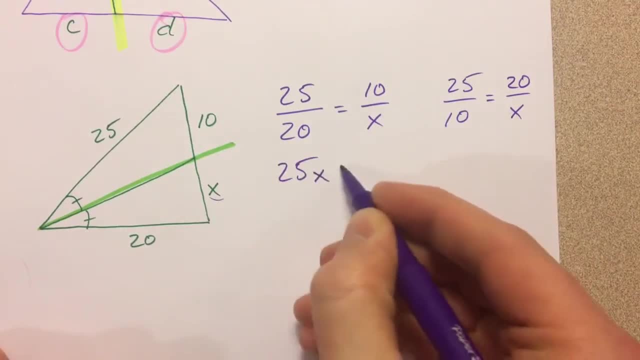 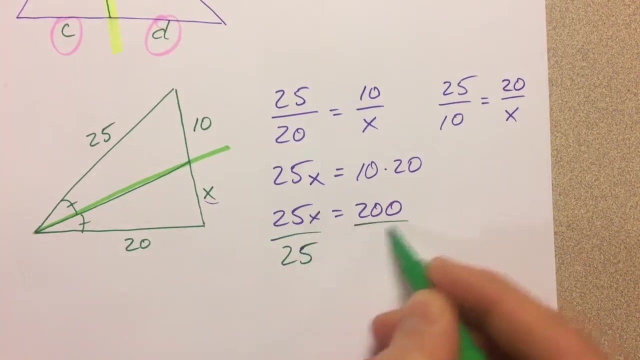 We cross, multiply, so we get 25 times X and we get 10 times 20,, which is 200.. And then we divide by that 25.. To get the X by itself, And 200 divided by 25 is 8.. 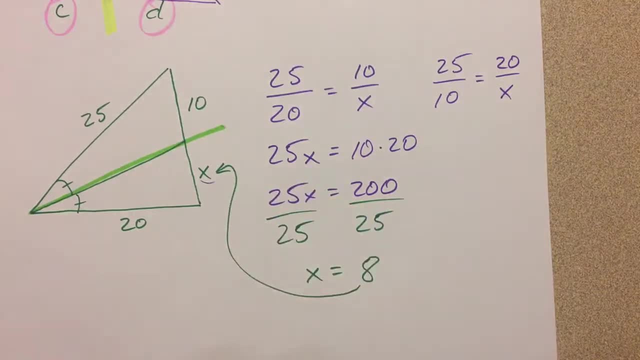 And so this 8 goes right there. And so that's the triangle angle bisector theorem. 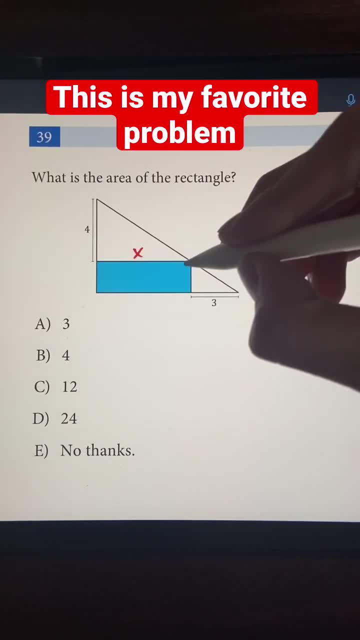 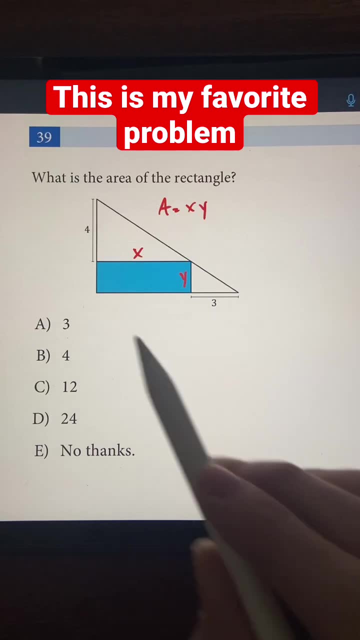 What is the area of the rectangle? I'm going to say that it has a width of some number x and a height of some number y, so that we know that the area is going to be equal to x times y. So now the next step is just to find x and y, and we have these two white triangles. so let's see if. 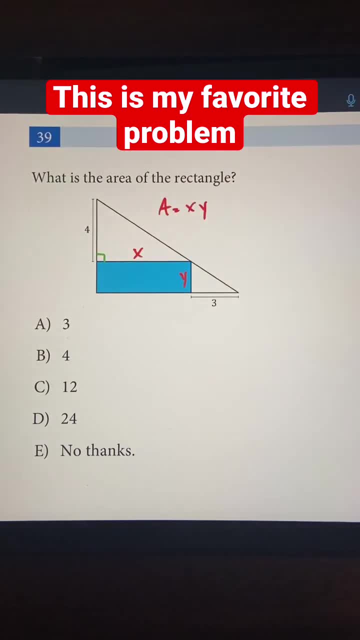 they are similar. So two triangles are similar if they have all of the same angles. So we have a right angle here, we have some angle right here and we also have an angle right here that is going to be the same in each of these triangles, which means these are indeed similar triangles. Take the